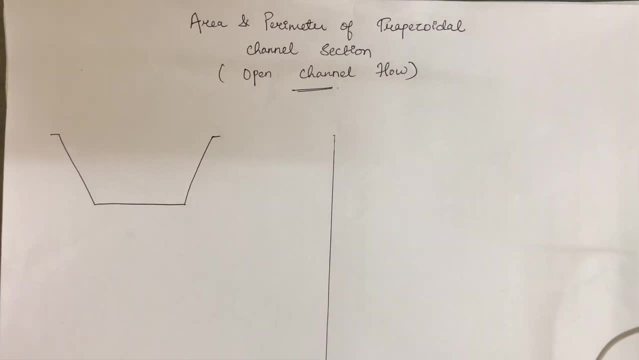 So, students, today in this video we are going to see that how we can calculate the area and perimeter of trapezoidal channel section, which will be very much helpful in the design of most economical channel section of open channel flow. So here, as you can see, a section of trapezoidal 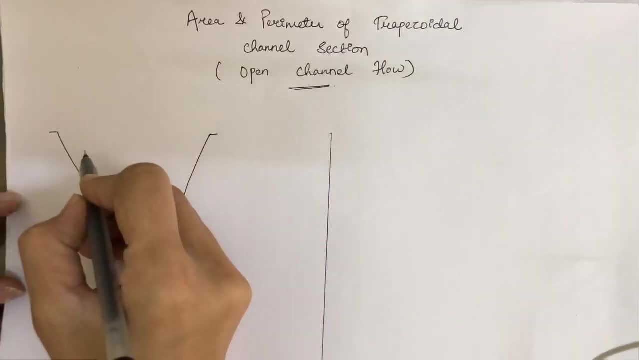 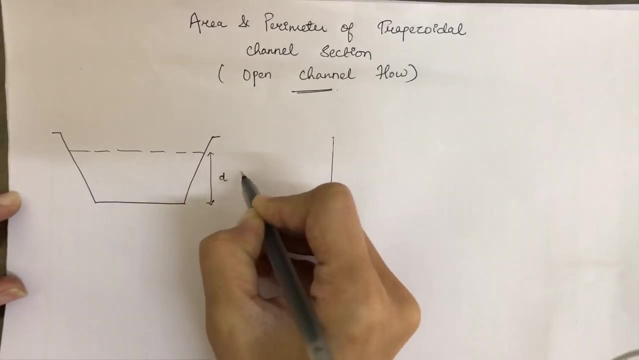 channel is shown, Let the depth of water which is present in the channel be represented by d. You can also use the other symbol, y, because in some books the symbol used is d, while in some books the symbol which is used to describe the depth of flow in an open channel is y. 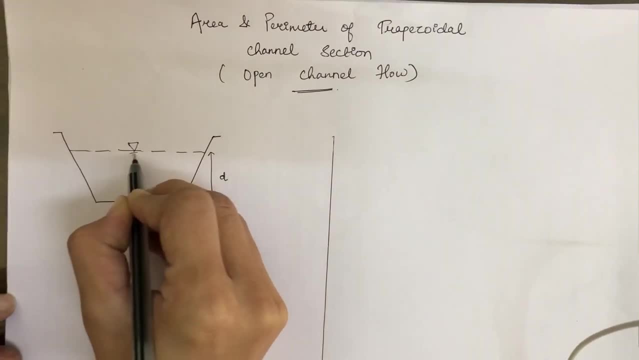 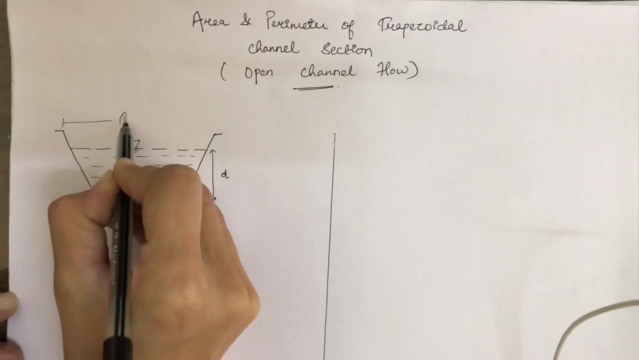 So this is the depth of flow in an open channel. or you can say this: much amount of water is present in your channel. Now let small b be the width of channel at the bottom and let capital b be the width of channel at the bottom. So this is the depth of flow in an open channel. 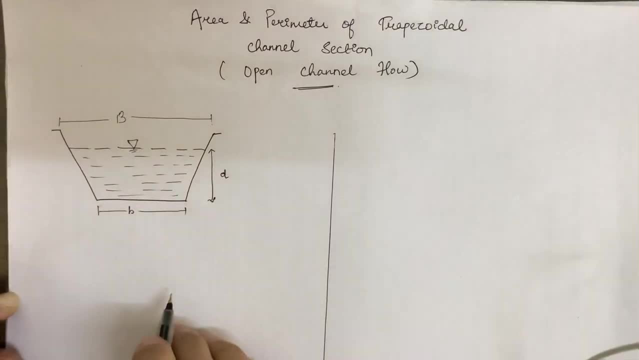 Now let capital b be the width of channel at the top. So here, as you can see in the figure, the top width of the trapezoidal channel section is somewhat more as compared to the bottom width of the channel section because of the side slopes. So let us begin with the first of all calculation. 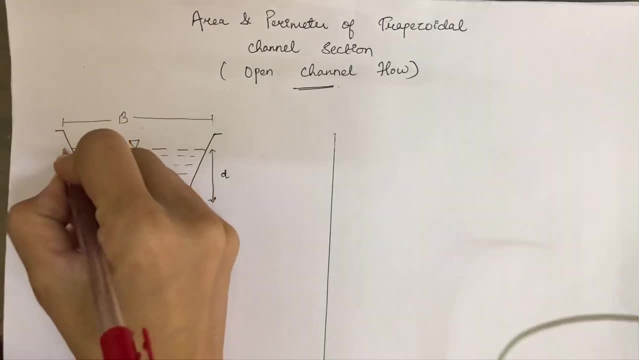 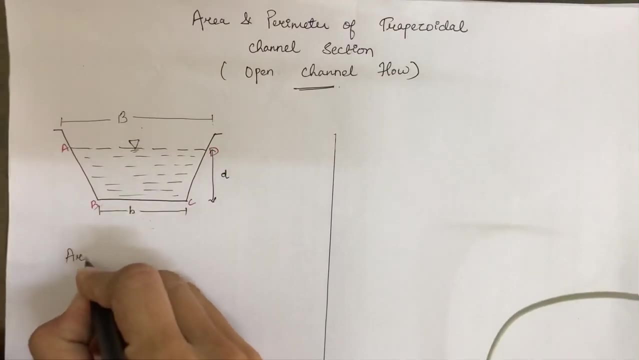 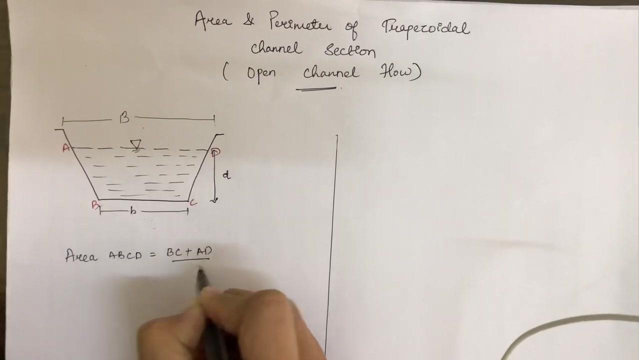 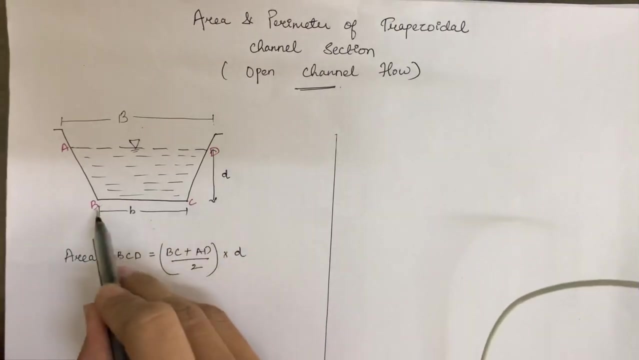 of area of this trapezoidal channel section. So, according to mathematical formula, the area of this channel section considering the water surface, ok, So it will be a, b, c, d, and that would be equals to b c plus a d by 2 into depth of flow. ok, So here, as you can see, the value of b c is: 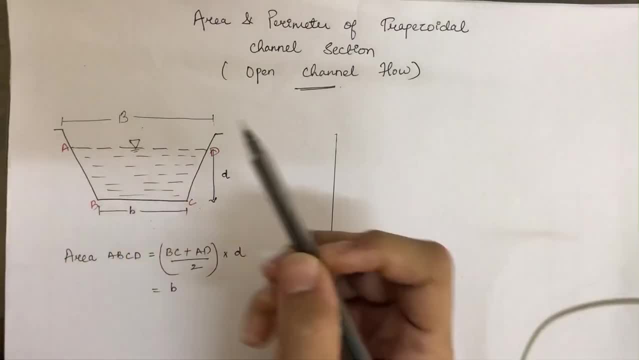 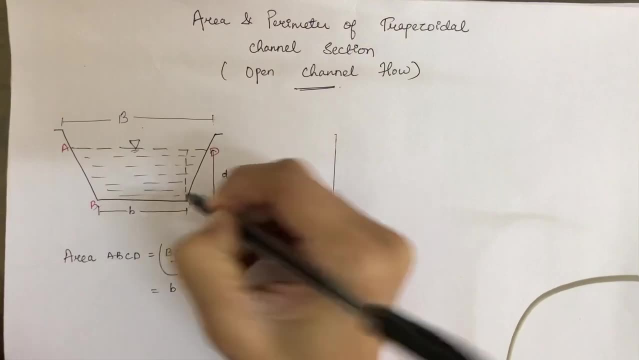 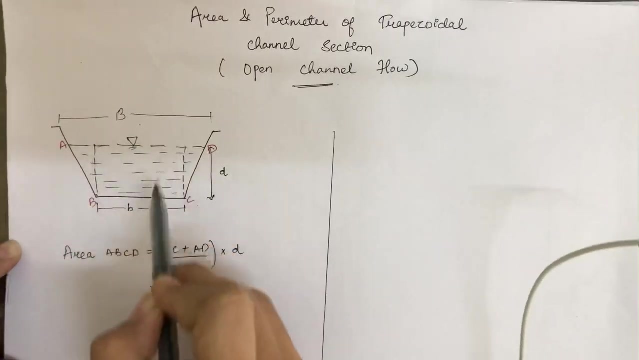 equals to small b and here, as you can see, a, d is the top width of the channel, which is capital. So if I make such sections on both these sides, then the top width would be equals to this much area, which is equals to small b plus this two remaining portion. ok, So it will be in the place. 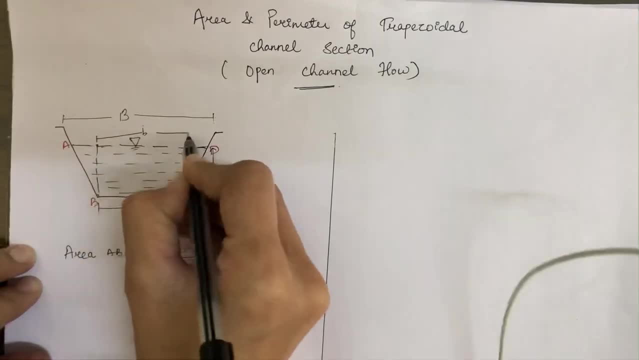 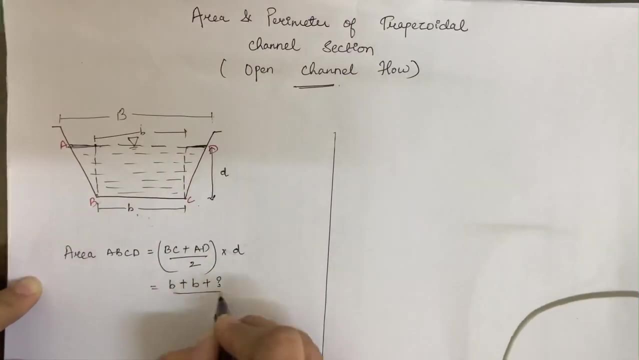 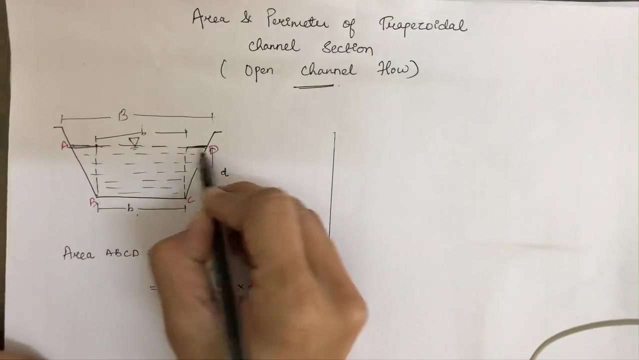 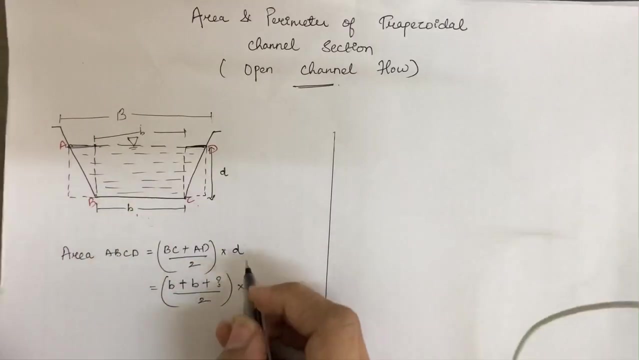 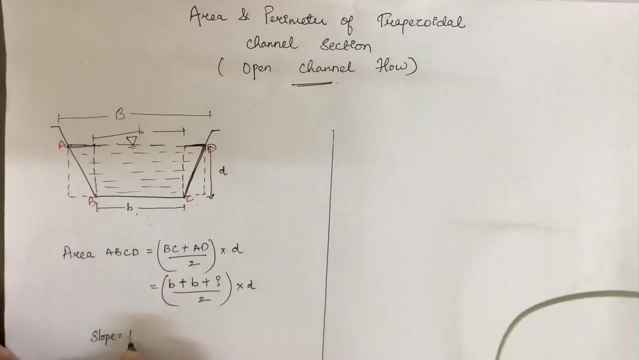 of a, d, I will write this: much is b, So b plus this two distance we need to find out. So that is question mark divided by 2 into depth of flow d. ok, So now, in order to find this depth. Ok, now we know that slope is represented as 1 by. 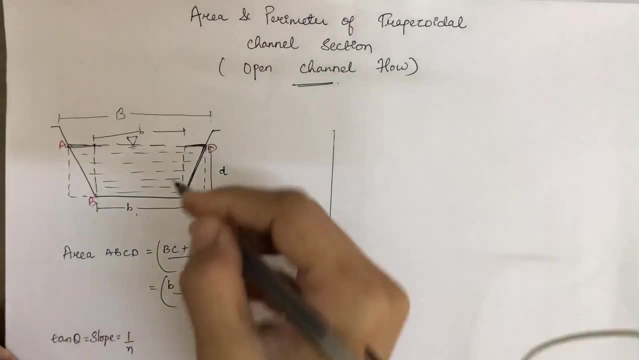 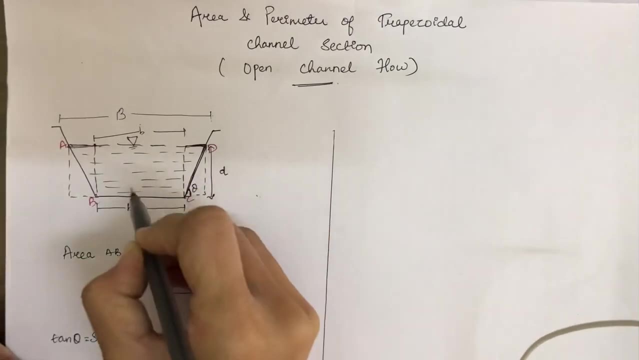 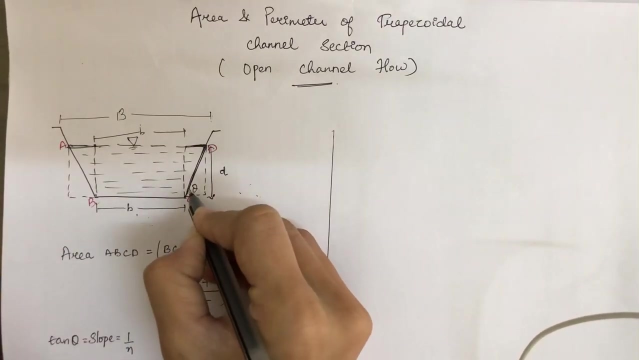 n and that is represented by 10 theta. ok, So here theta is the angle which this slope of the channel is making with the horizon, or you can say with the bed slope of the channel or width of the channel. So here, as this: 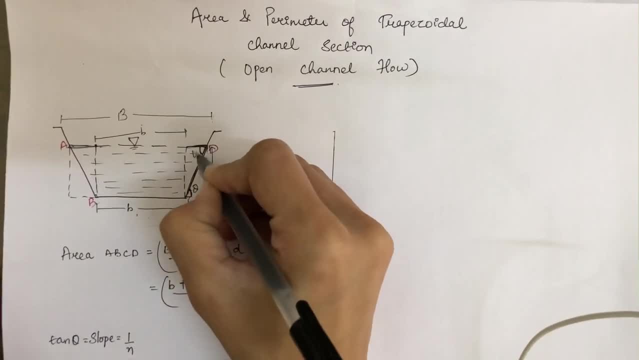 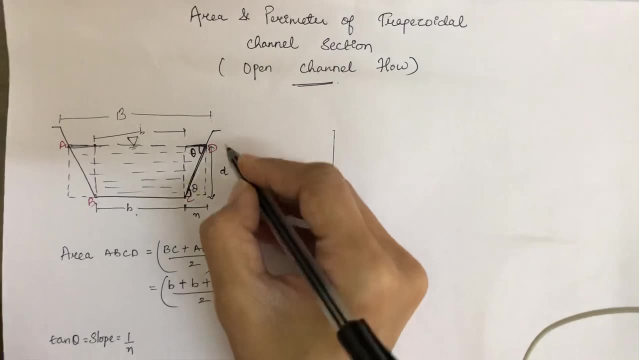 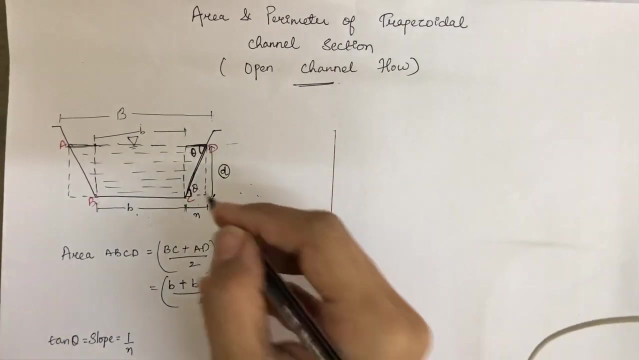 angle is theta. according to mathematical roots, this angle must be equals to theta, and this is represented by n, which is horizontal, and this is represented by 1, which is vertical. but here, in this case, we are taking d, So here I will give this point the value. 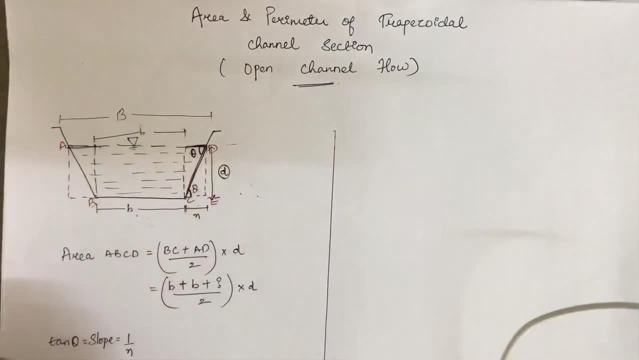 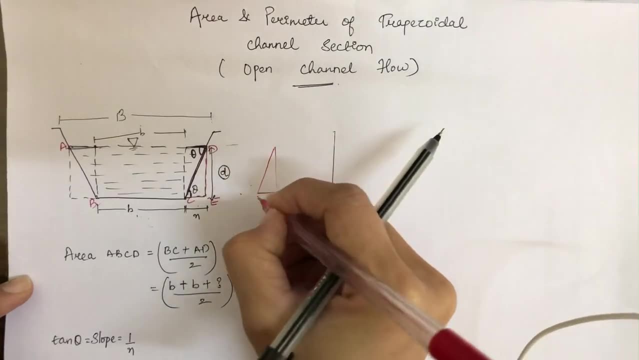 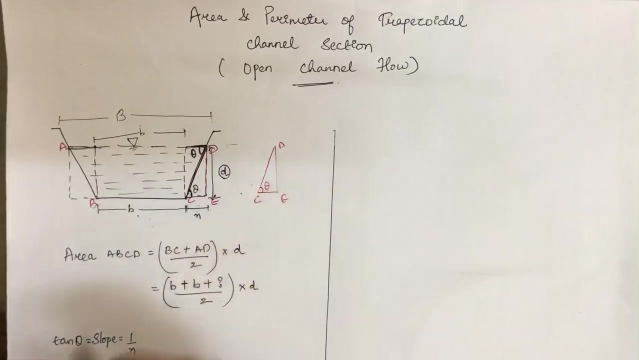 of c, e, ok, So if in this triangle- ok, this triangle I am making here again- So in this triangle c, d, e, this is theta. if we apply the formula of 10 theta, ok, which represents slope, So 10, 10 theta, 10 theta is equals to you. 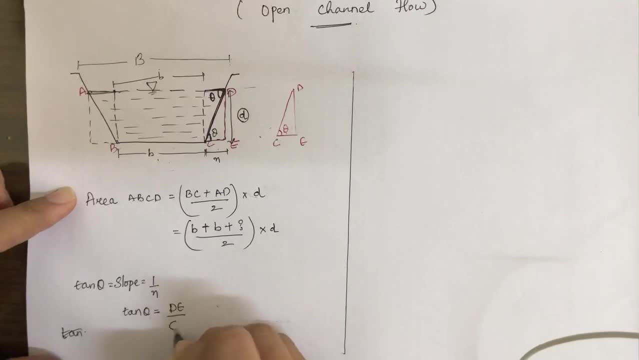 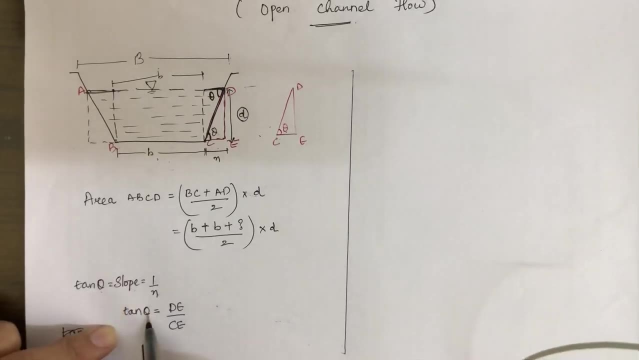 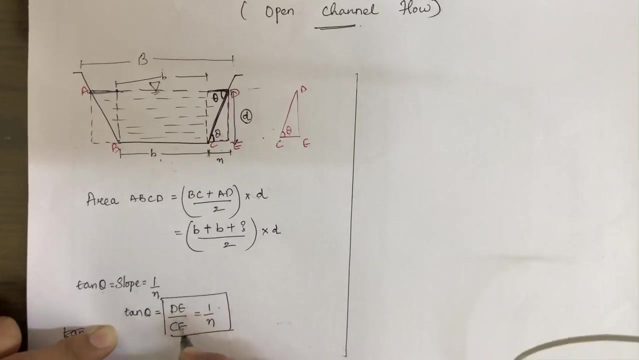 to opposite upon adjacent, that is, d? e upon c? e and tan theta is nothing, but it is equals to slope and it is its value is 1 by n. so in place of tan theta i will write 1 by n. ok, so this is: 1 by n is equals to d? e upon c? e is equals to tan theta. so if i want the 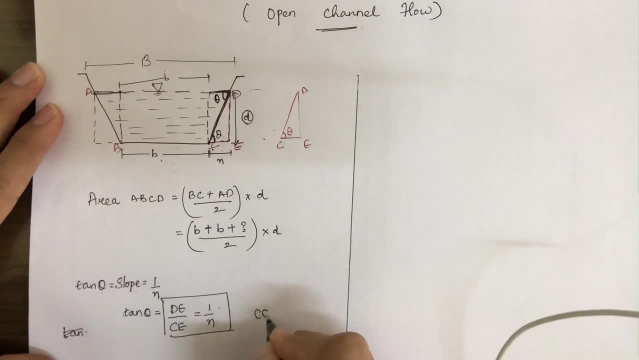 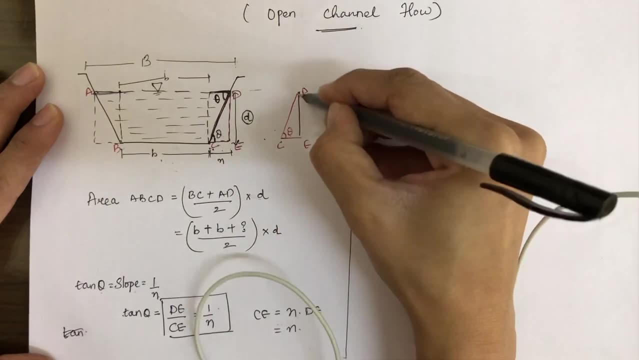 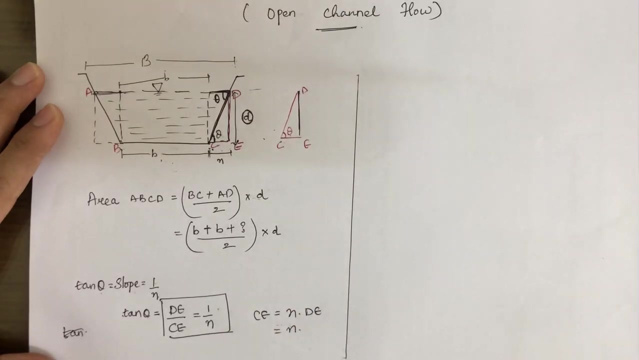 value of c? e, then it will be: c? e is equals to n into d e is equals to n into d? e is what here? in our case d? e is depth of flow, which is represented by small d? ok. so in that case, d? e will be equals to n? d and the value of c? e is equals to n? d ok. so as this value is, 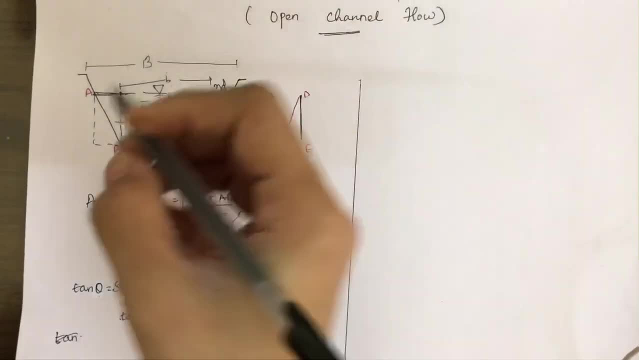 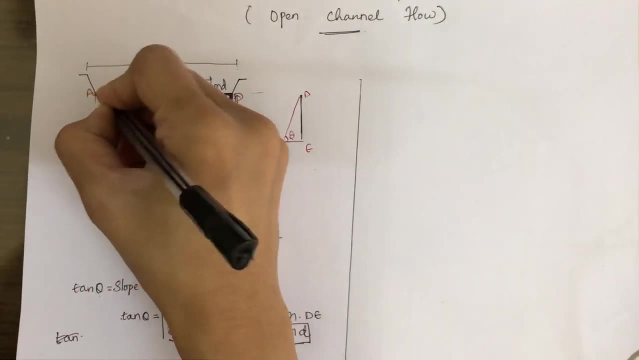 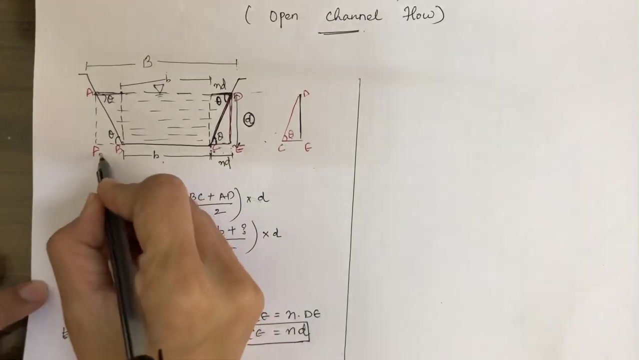 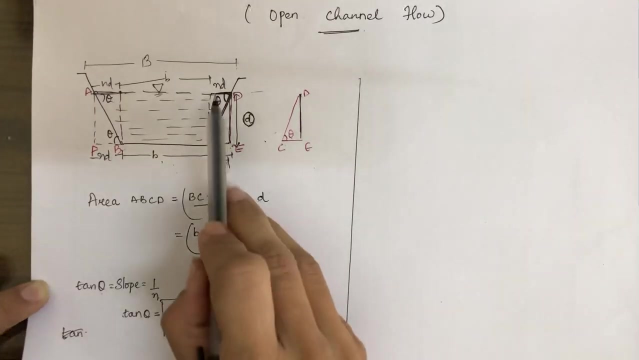 n d, This value will be equals to n d. again here, if i give a point f, then an applying similar equation: this is theta, this is theta. so again, this will be equals to n into d and this will be again equals to n into d. clear. so here now we got the value of this two portions. 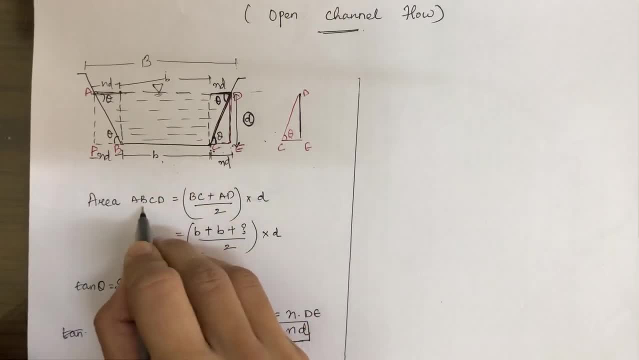 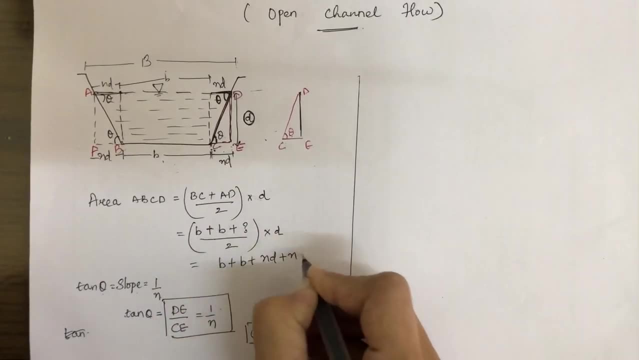 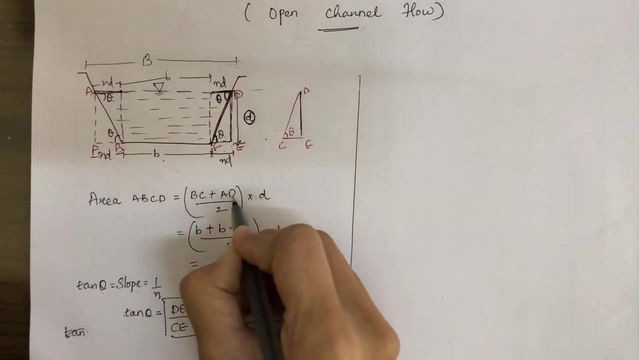 as n d and n d, so again substituting that value In our equation. so it will be b plus b plus n d plus n d, this two portion. so we will get the entire length b, which is equals to a d. so in place of a d it will be b plus n d plus. 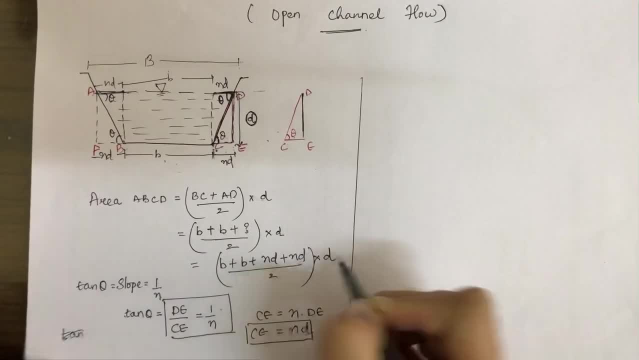 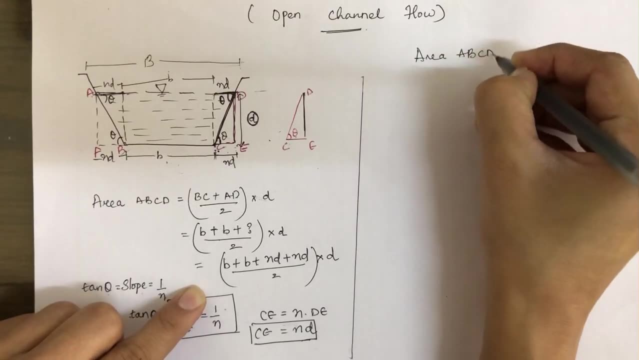 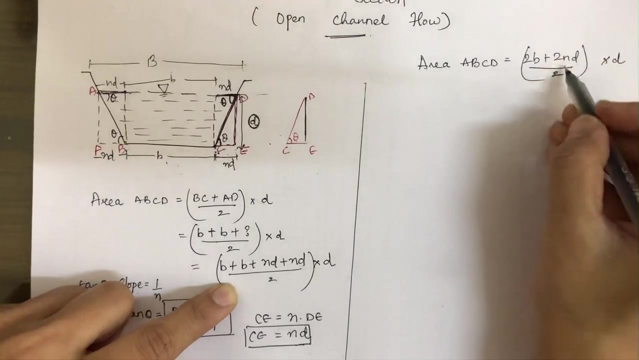 n, d divided by 2 into d. ok, so your area a, b, c, d will be equals to 2 b plus n d divided 2ND by 2 into D. taking two common, so 2B plus ND into D by 2, 2, 2, cancel out. so. 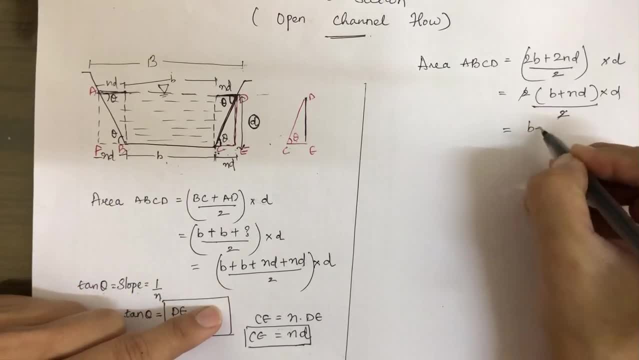 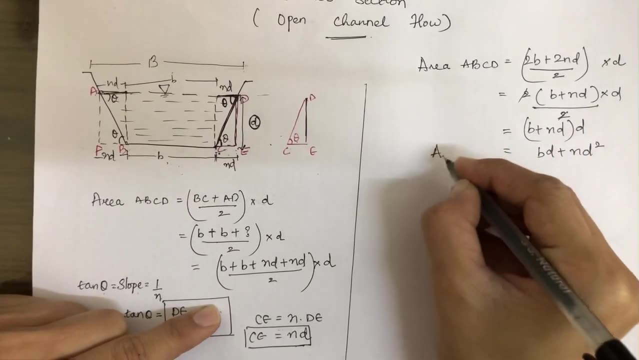 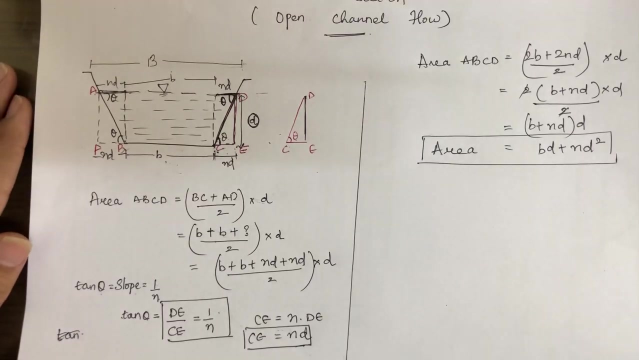 the value of area ABCD will be B plus ND into D, or you can also write BD plus ND square. So this is the area of trapezoidal channel section in case of open channel flow clear. Now we will move towards the second parameter, that is, the 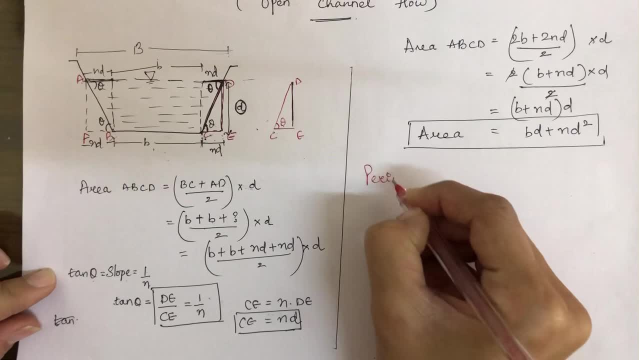 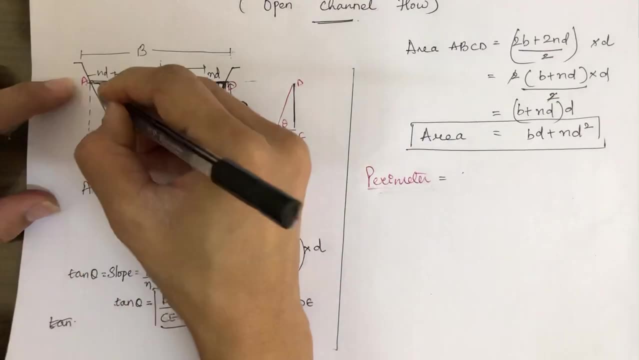 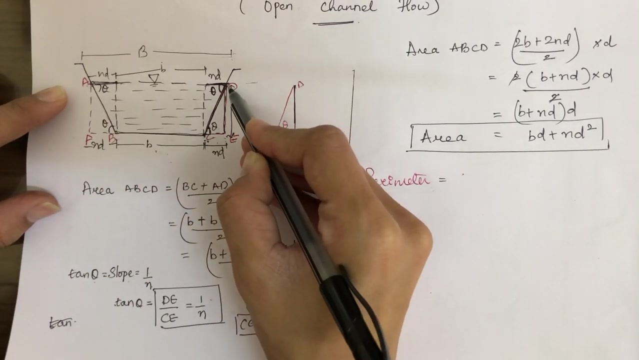 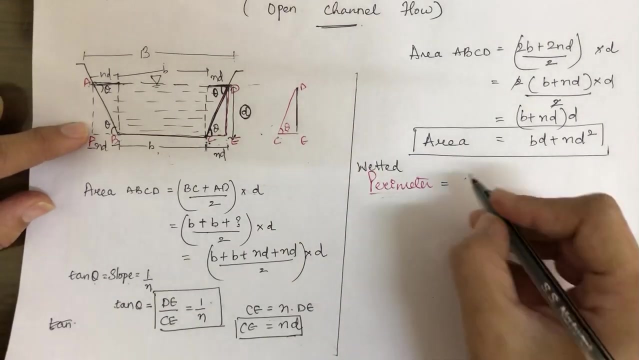 perimeter. So here, in case of perimeter, what will be the total value? it will be equals to this: AB plus BC plus CD. okay, and sorry, here I should write precisely wetted perimeter. okay, so the wetted perimeter would be AB plus BC plus CD. this much.